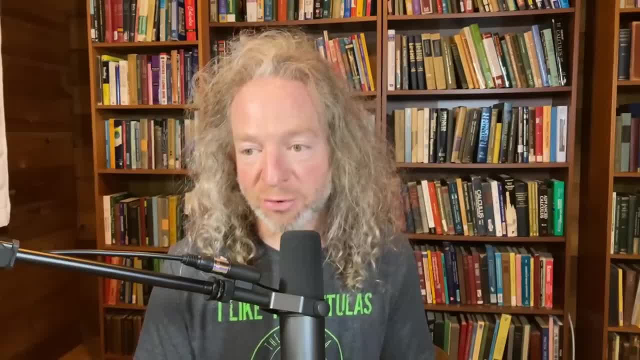 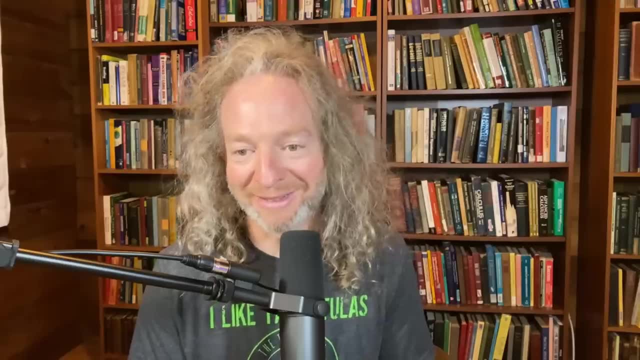 that would be great for someone like me who's just starting out with proofs in linear algebra. I know your suggestions would be like a treasure map leading me to mathematical enlightenment. Your content has been a game changer for me and I'm genuinely grateful that you're watching this video. I hope you enjoy it And I'll see you in the next video. 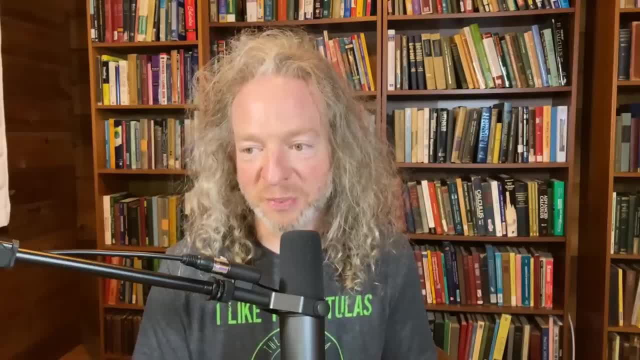 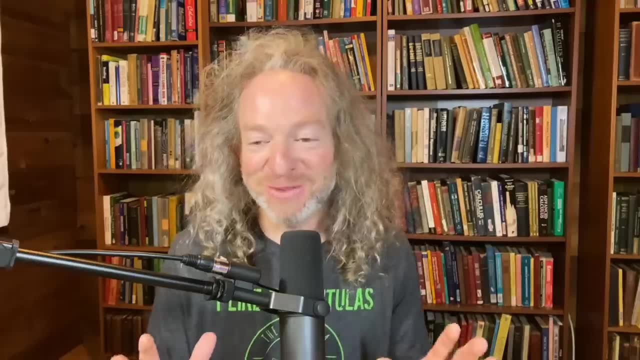 for the passion and enthusiasm you bring to math education, Looking forward to your recommendations and I'll eagerly be watching your next video. Best regards, Amir. So first let me just say two things to this message. So thank you, Amir, for sending this. 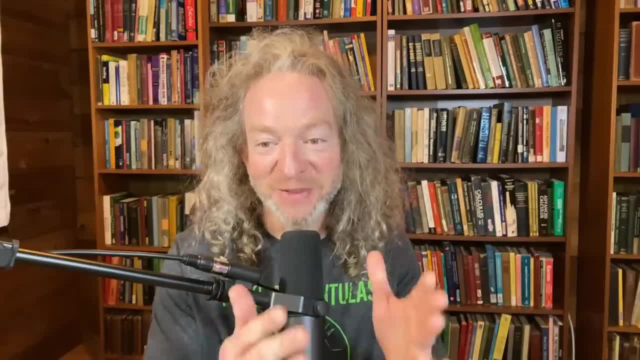 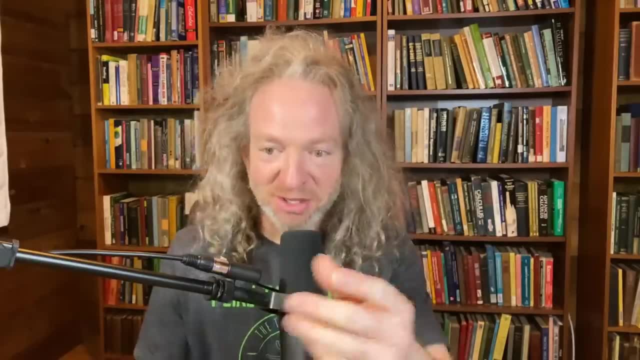 message. And secondly, I think it's really funny that you said it's the first time I'm encountering proofs in math, because the truth is, I had not read this email until right now And it just basically agrees with everything I just said. So I feel like what's the word I'm looking for? 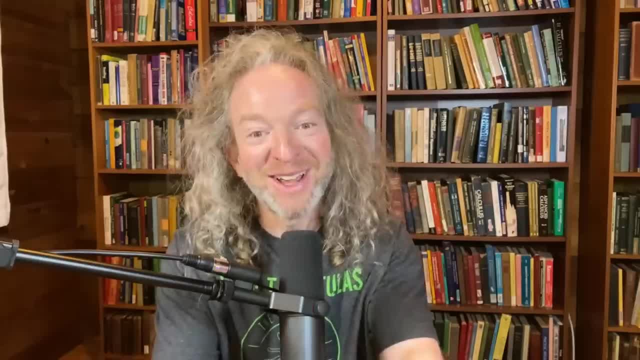 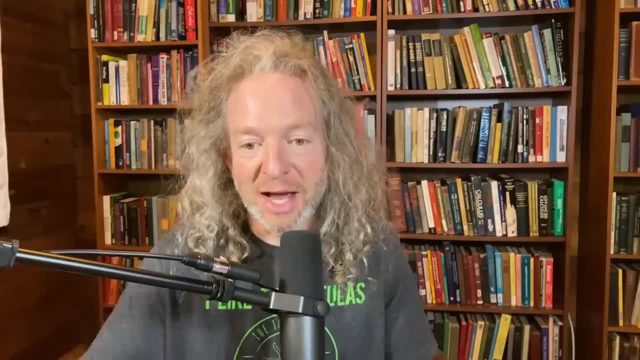 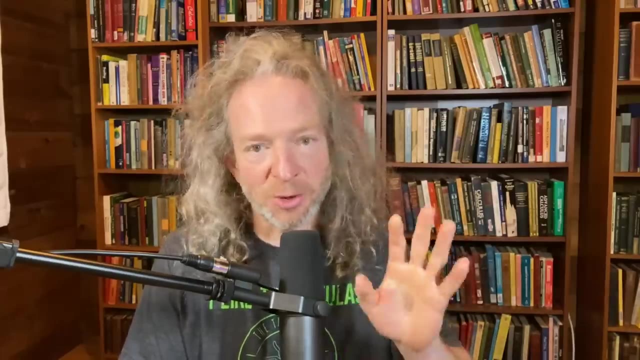 Validated? Yes, So for many people, including Amir, it is the first time that they see proofs. So I do have two recommendations, And I think my first one is one that anyone watching this video who wants to learn linear algebra should take. It's a no-brainer because it's a book that is widely 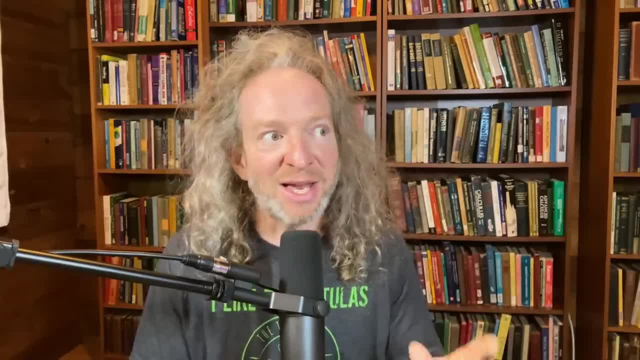 available. It's super affordable if you can get used copies And in my opinion it's one of the best books for linear algebra. You might not feel that way if you're using it for a course, but if you compare it to a lot of other books, it's a good book And I think it's one of the best books. 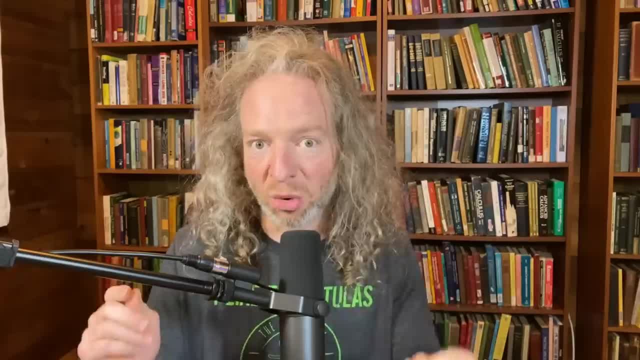 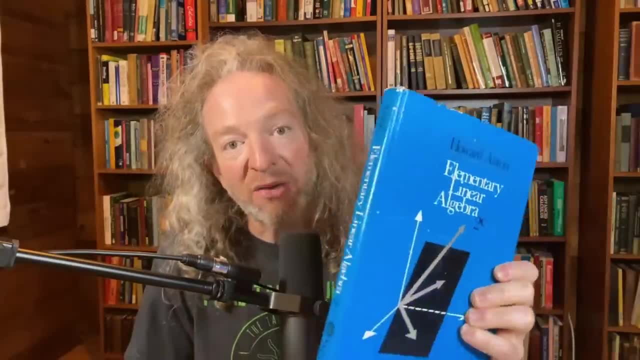 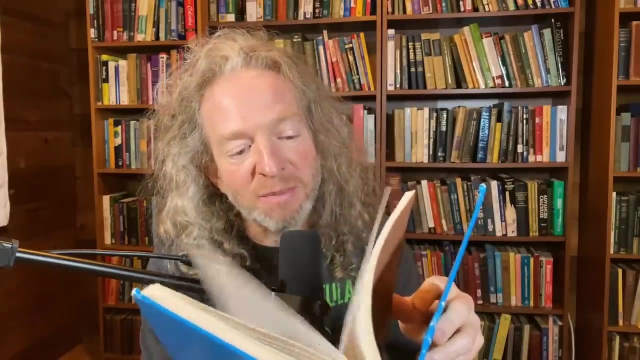 out there. This book is gold. It literally is like a treasure. It has withstood the test of time. Here's a really old copy. This is the second edition of Howard Anton's Elementary Linear Algebra. This is the classic book on linear algebra And one of the best things about. 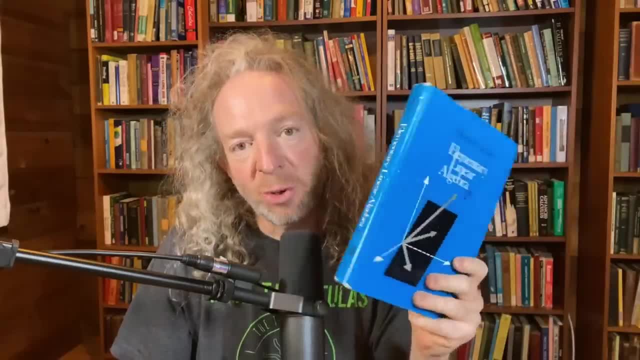 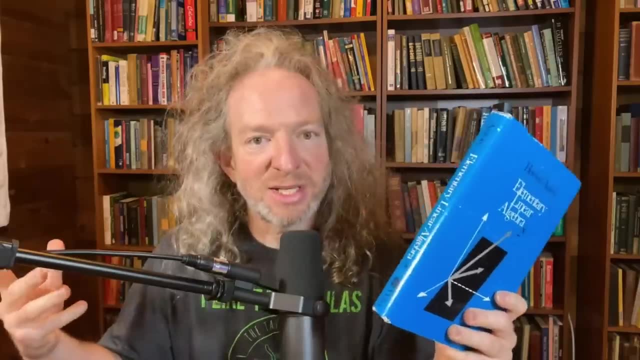 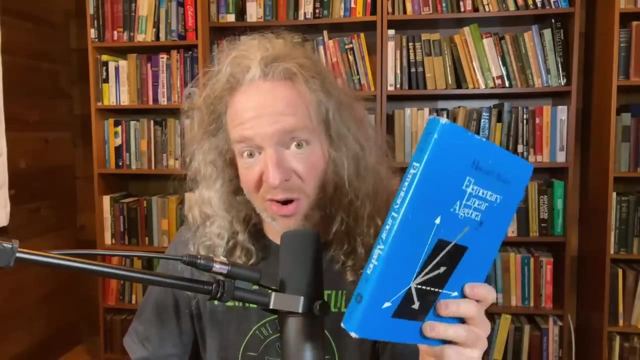 this book is that it's very modern, Even though it's an older book and it's been reprinted several times. the content in this book is content that is timeless in a sense. If you're taking linear algebra and you're taking a class and you're not using this book, well, chances are when you have. 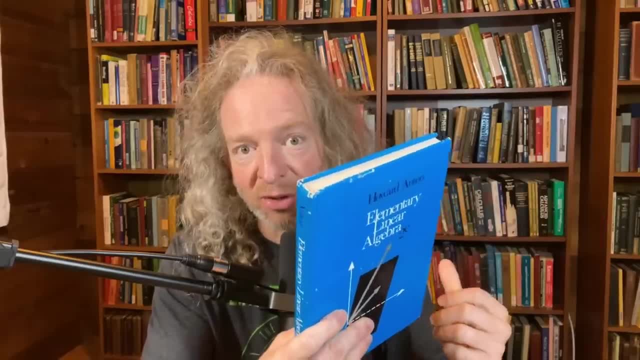 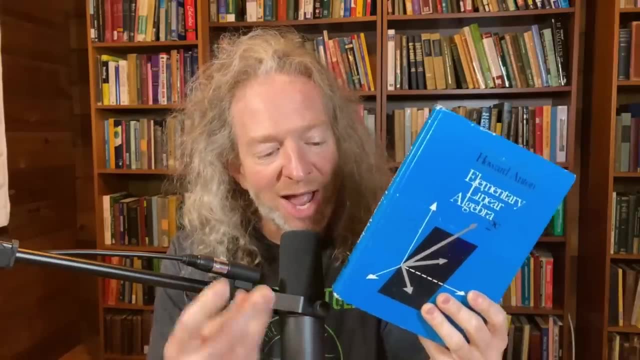 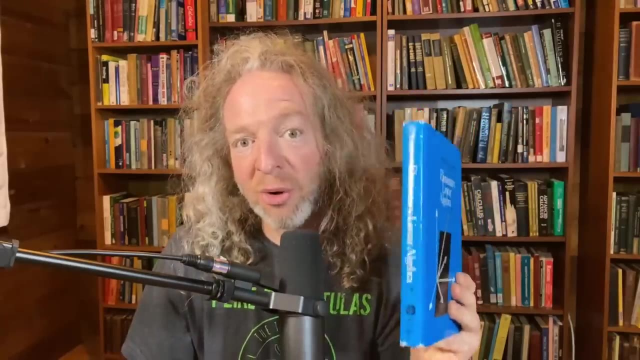 a test. a lot of your test questions will be very similar to the questions in this book because it's very, very standard. A lot of the flavor of the questions and the way they're asked and the types of questions they're things that you often find in this book, So it's a great resource for extra. 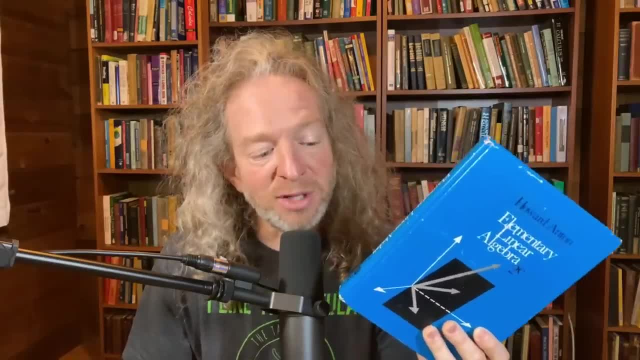 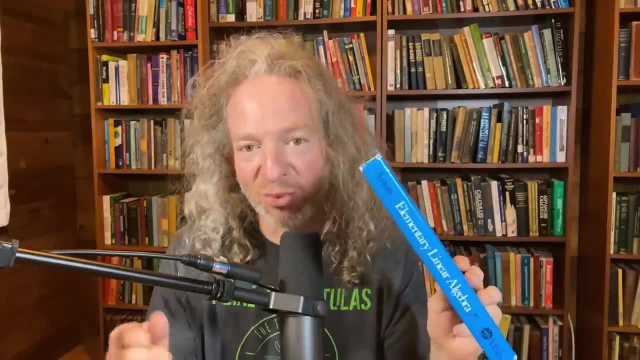 practice problems, And I think that makes it probably the best learning tool for you. Thank you so much for joining me today. I hope you enjoyed this video. I hope you enjoyed it And I'll see you in the next one. Bye-bye. 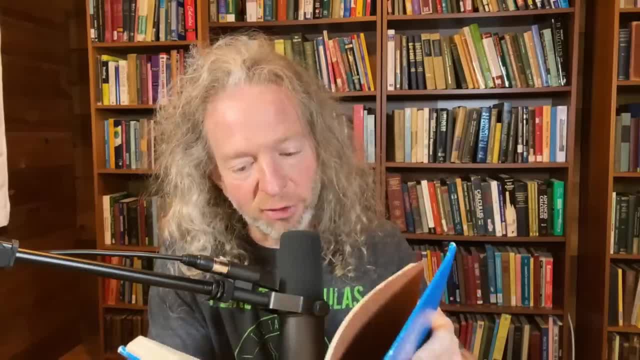 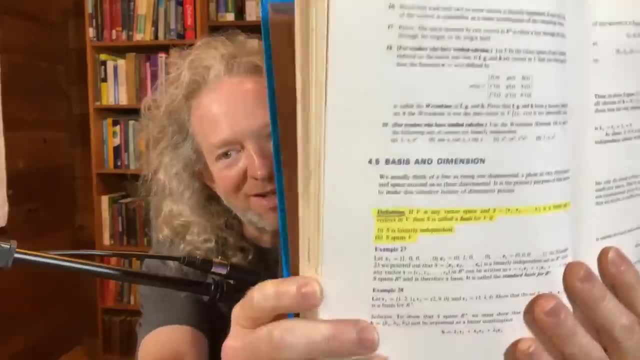 Awesome book. I should probably do a video where I do a full, careful review on this book, because it's just got so many good examples. Yeah, Basis and Dimension. Look at that. Someone was studying Basis and Dimension there. You see the layout. See how the layout is very modern. It's just a. 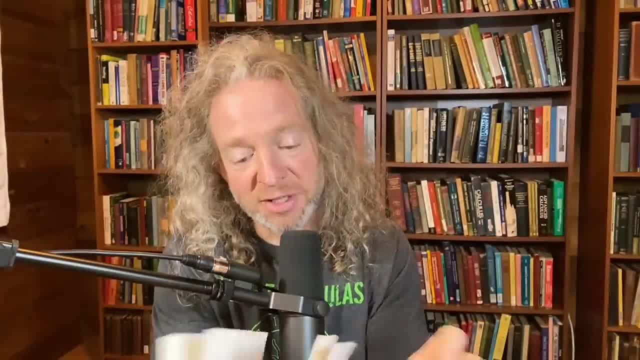 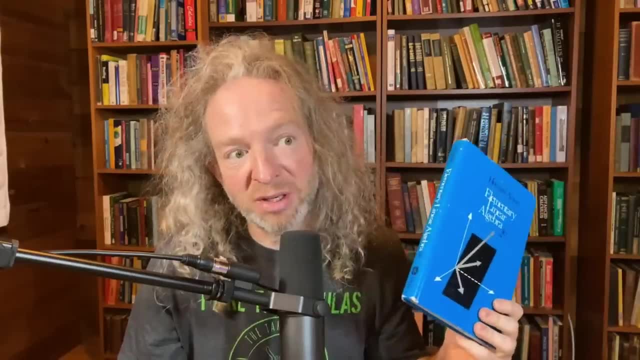 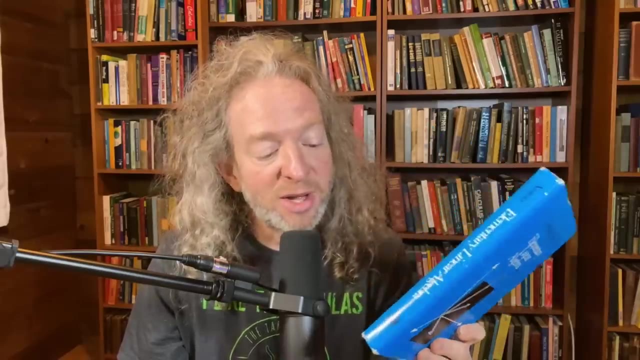 nice, clean book, Very, very good. And as much as I love other books by Serge Lang and Hoffman and Kunz- a lot of the older classics- Anton's book has really withstood the test of time for a reason: It's easy And it'll help you learn linear algebra. Now it does have some proofs. 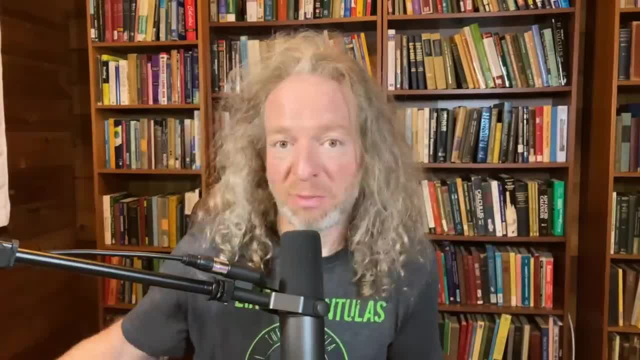 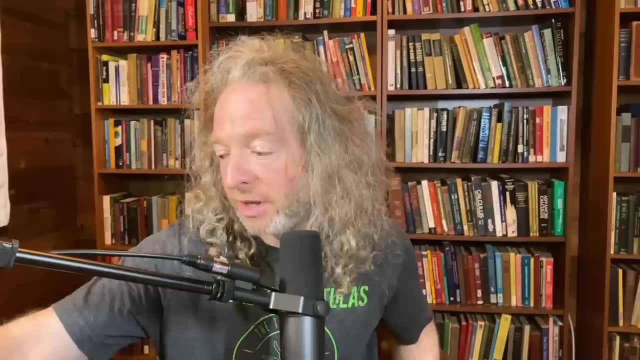 but it is not a proof-based linear algebra book. For a proof-based linear algebra book, normally in the past people would use Hoffman and Kunz- And you can still use that one, And I was actually just looking at that one this morning for another reason- But a more modern. 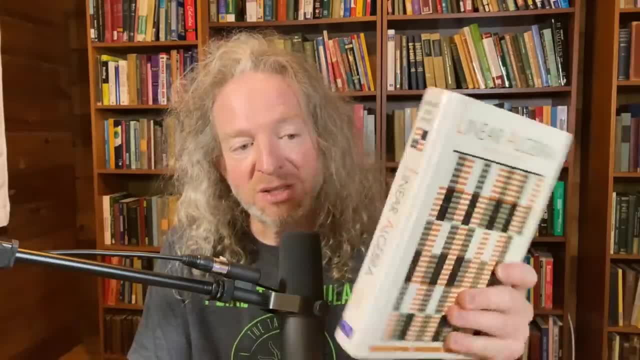 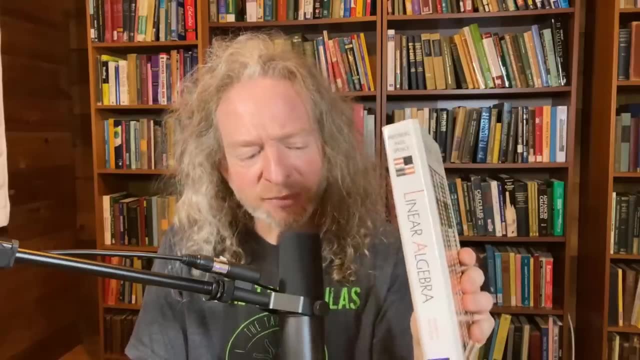 approach would be the one by Friedberg, Inzel and Spence. Not only is this a more modern take on linear algebra- just the layout of the section And the way it's written, it also serves as an excellent reference. So when you go further in, 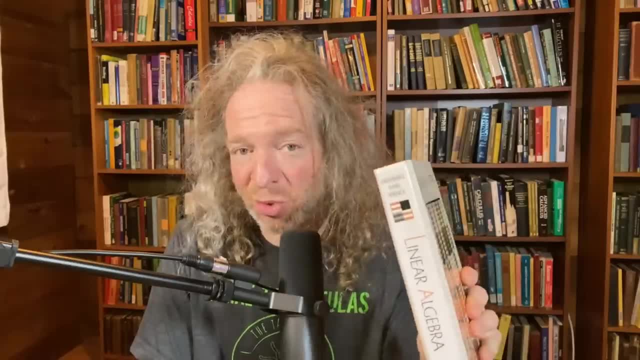 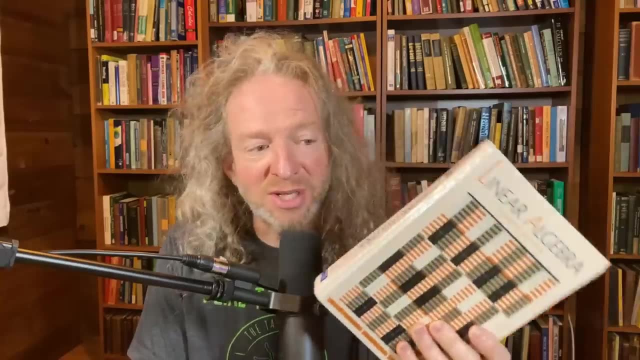 mathematics into other classes, even classes in graduate school. you might forget things and you might have to look them up, And this is a great resource because it serves as a great reference Again. this is another, I think, must-have linear algebra book for any one series. 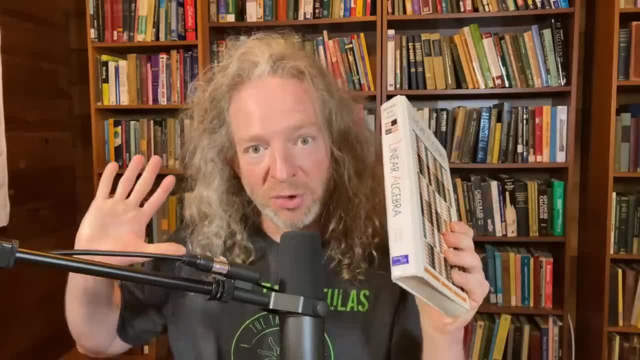 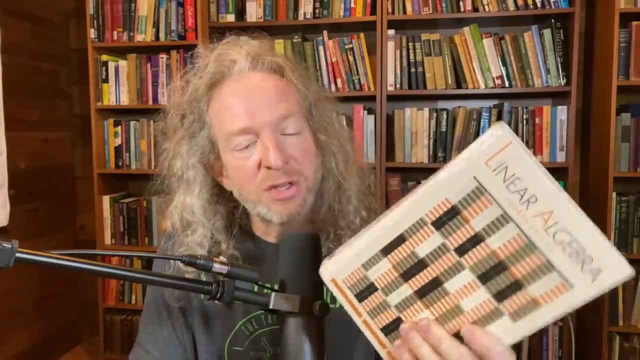 about mathematics. So these two books are, I think, gold Treasure Map. that's it. So this book caused me a lot of pain When I learned linear algebra, so I used this book for an actual course, a second course on 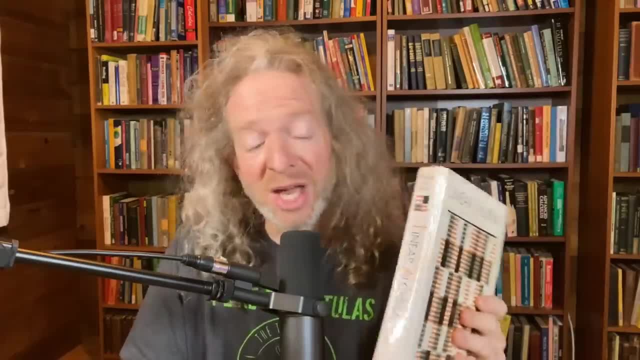 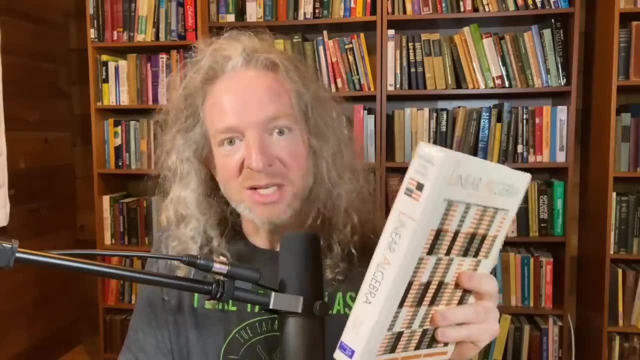 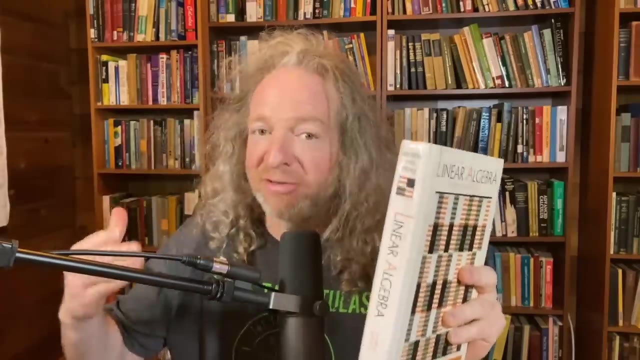 linear algebra, a course in which I did not get an A. I actually got an A minus in here, And it's because I didn't learn the material well enough. I deserved the A minus. I definitely did not deserve an A. I don't like the word deserve, That's a whole other video, But I definitely. 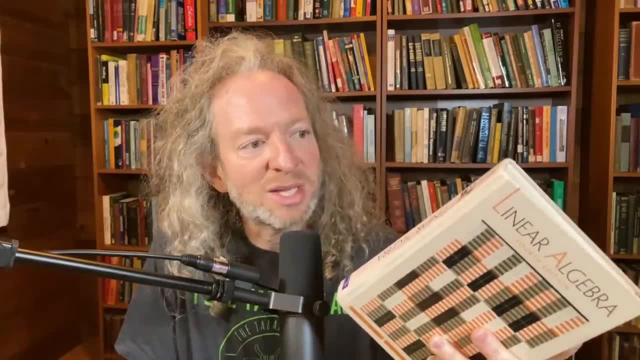 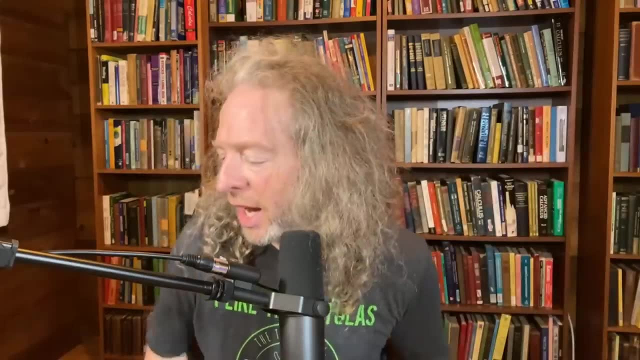 did not deserve an A And I got an A minus And I think it was well-assigned and well-earned. This book is hard, It has proofs and the proofs are very rigorous And, honestly, I always think that you get to a. 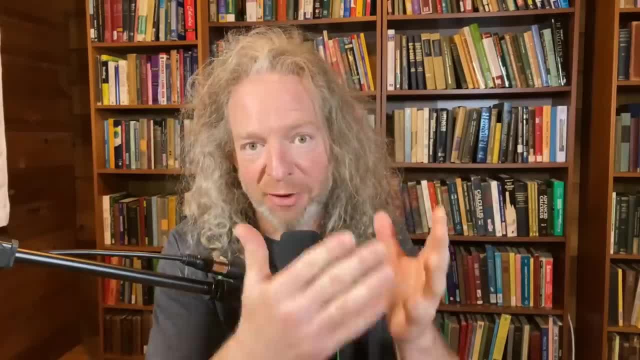 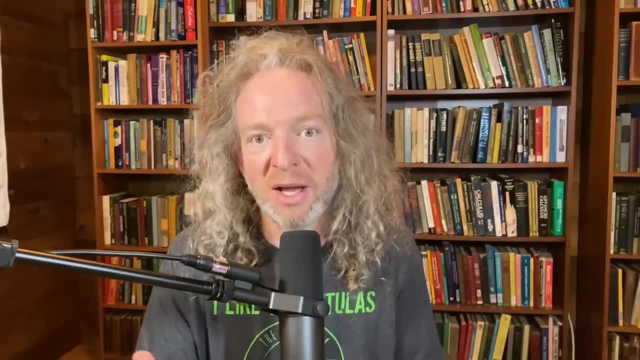 point in math where, whenever you write your own proofs, they're better than the proofs in the book, And that's because your proofs are easier to understand than someone else's proofs. It's like programming: If you're looking at someone's program and you're trying to read their code. 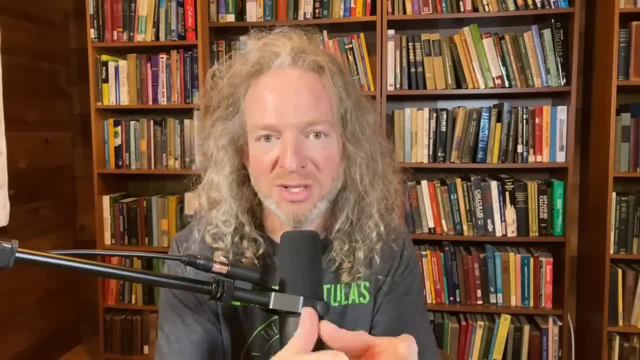 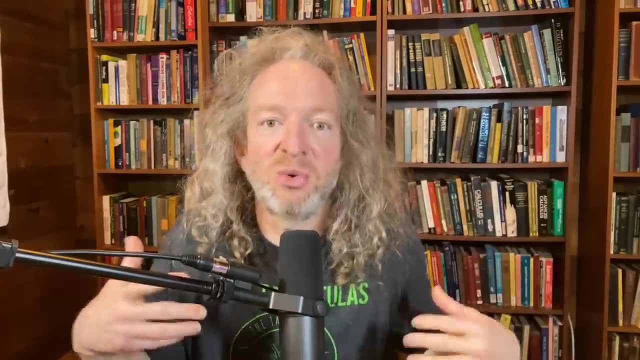 that's much, much harder than reading your own code. Same thing with proofs. right, Reading someone else's proof is harder than reading your own, because you kind of have to figure out what they did. If you write your own proof, you know what you did, because you already constructed that logical. 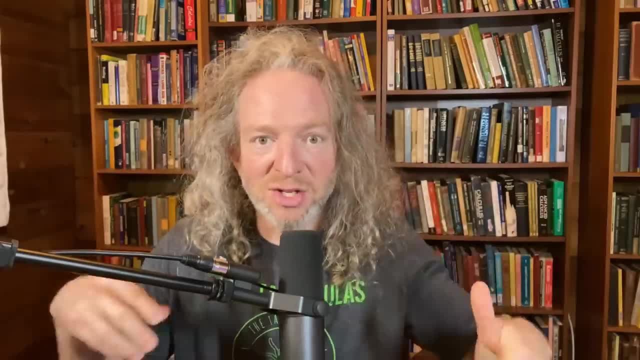 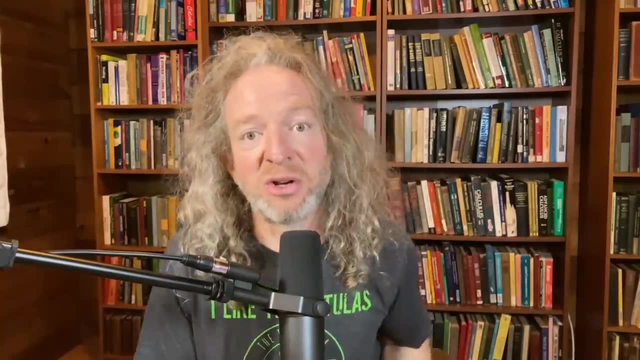 chain of thoughts to get to the conclusion You know everything already, so you're just kind of validating what you've already done, Whereas if you're looking at someone else's work, like in this book- here you're looking at a proof in this book. you're kind of looking at it and thinking: 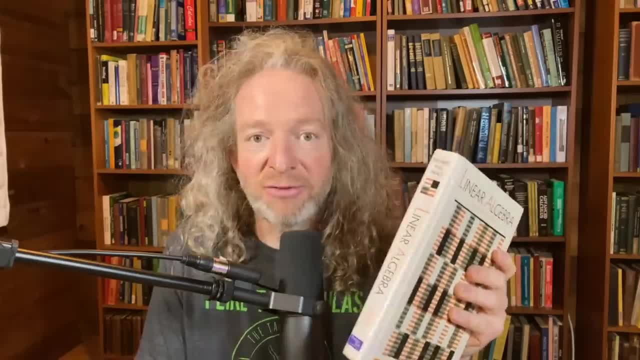 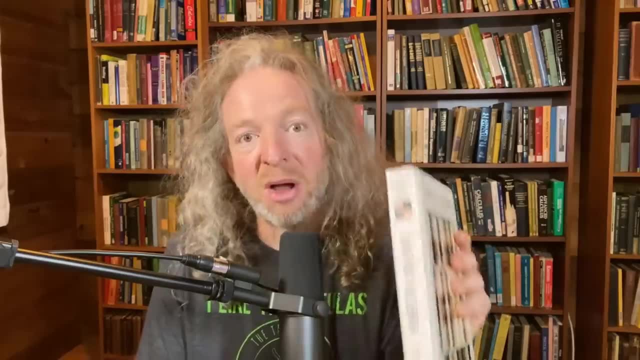 oh, what did they do? So one piece of advice I have for you on proof writing and linear algebra, because you mentioned that- is that whenever you're working on mathematics- any mathematics from any math book- always try to do the proofs on your own first. 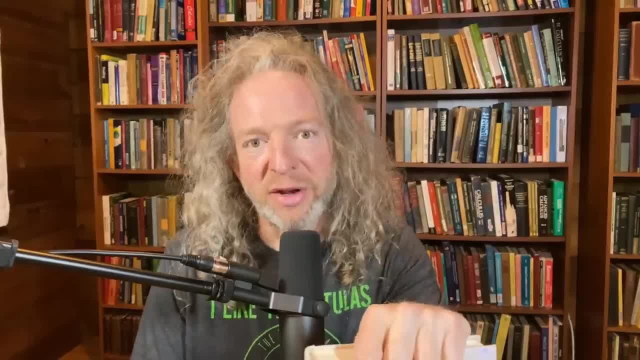 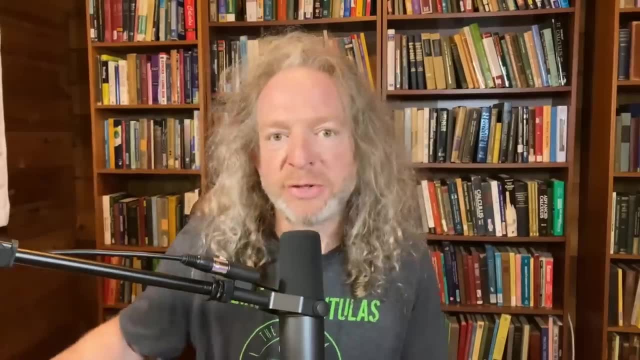 You know it's a well. it's well worth it. I had a friend- he's still my friend, I don't know why I said had- and he took an entire summer and he read Rudin's Principles of Mathematical Analysis and he 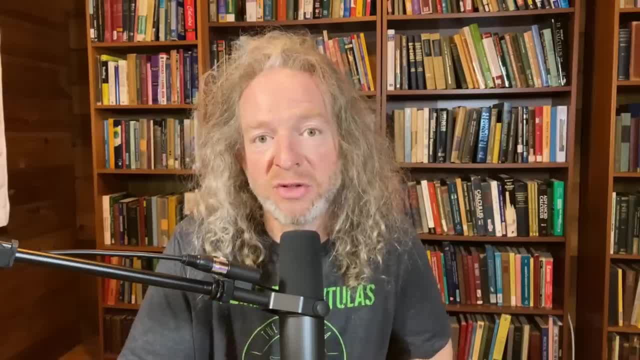 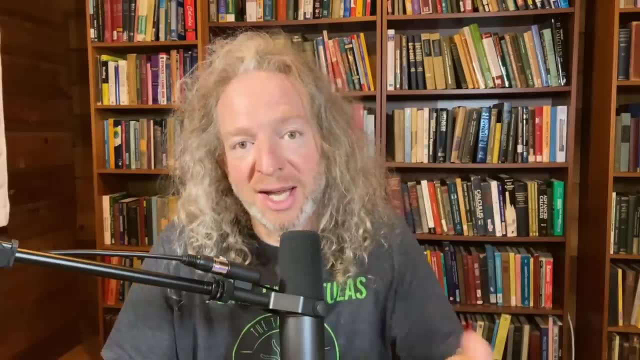 didn't do the exercises, but his strategy was he would go through all the examples and he would try to do every proof and every example on his own before you know, looking at the book before looking at the solution in the book. And that's a good attempt. Was he able to do it? Obviously not. 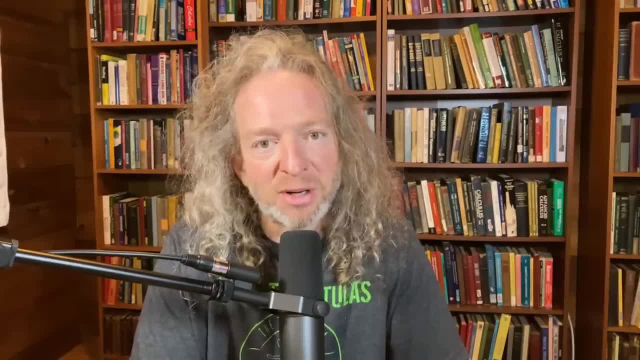 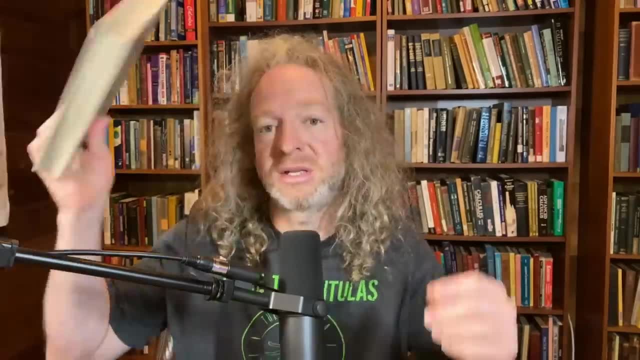 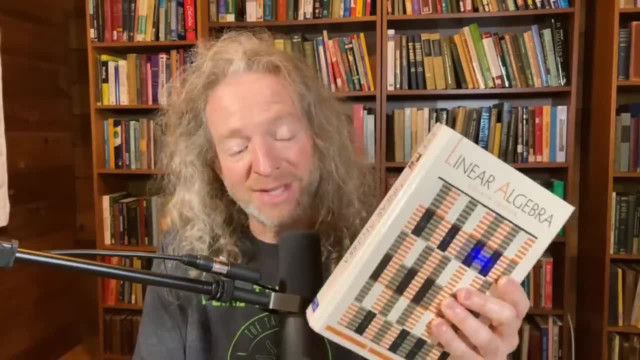 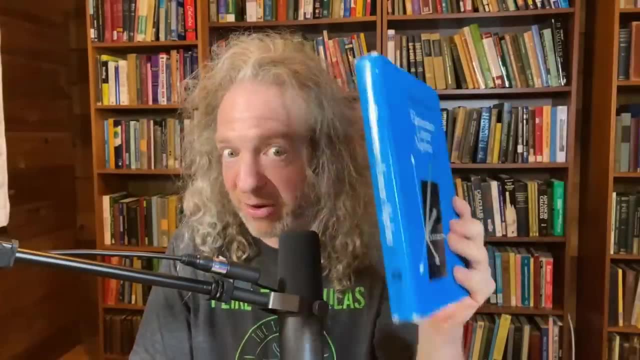 do the best you can. It's not a perfect book. It's definitely much harder than this one, So this is one. this is one for beginners- Again, the one by Anton, definitely for beginners. Very good book. I like this one much better than the Freedboat book. Nothing against these amazing authors and 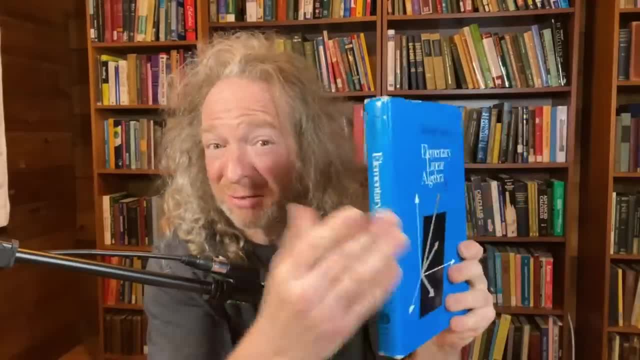 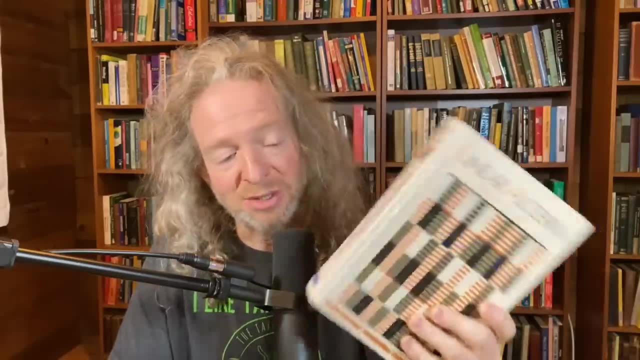 amazing mathematicians. This is just an easier book, right? This is for beginners. Anton's book is for beginners, whereas this is meant for people who have already had a proof writing course, So well worth getting both. though Two very different levels of linear algebra: There's a 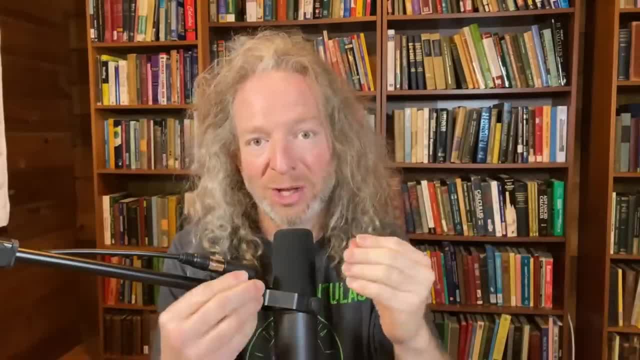 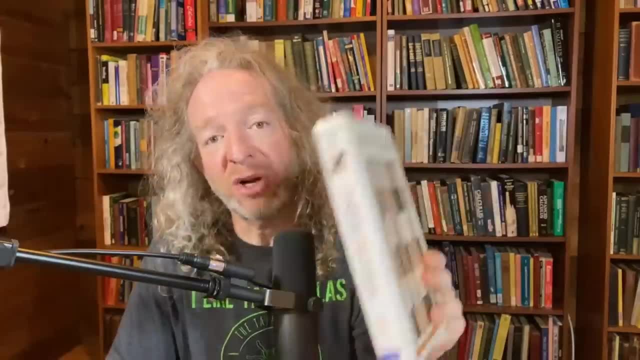 very big difference in the way the books are written and the way the proofs are written, but both of them are worth having. And the Freedboat book, I learned to appreciate it after I took the course, So after I took linear algebra and got my A minus and moved on with my 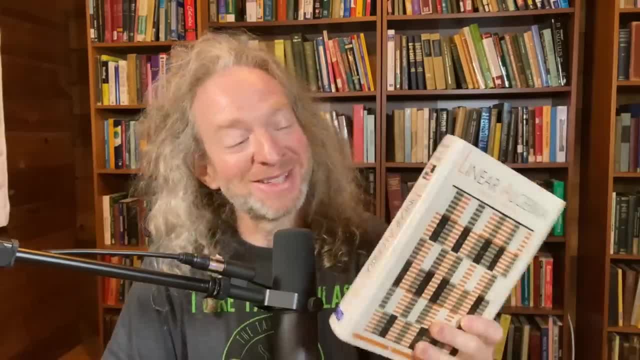 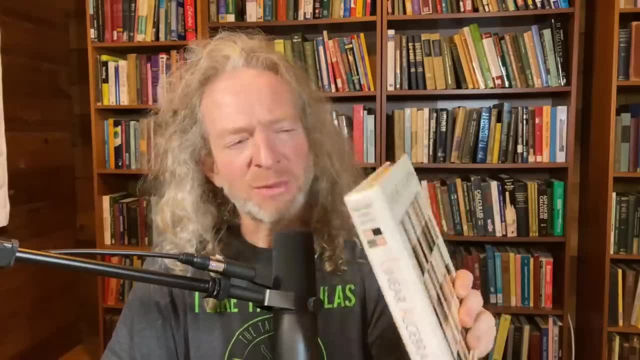 life and I make it sound bad. I was very happy with the A minus. I did end up referencing this in graduate school because I studied quite a bit of linear algebra in graduate school And I remember looking up stuff like regarding the minimal polynomial and certain 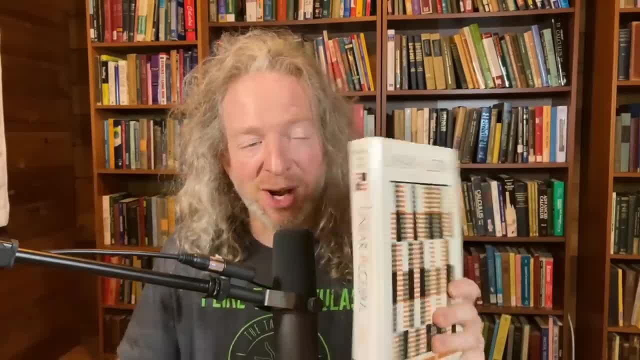 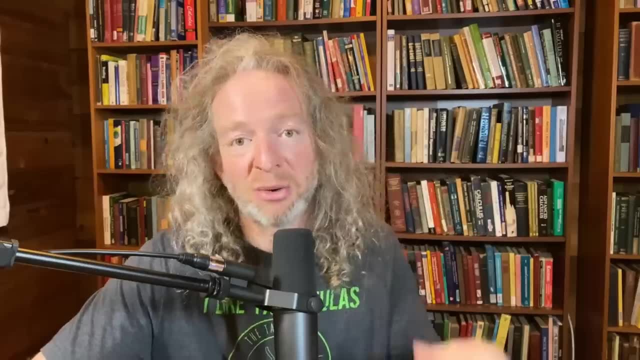 theorems that I perhaps didn't cover or forgot as an undergrad, So it helps to have this book on your bookshelf. I'll leave links in the description to both of these books, Amir, in case you want to check them out or in case anyone else wants to check them out. And linear algebra is tough. I. 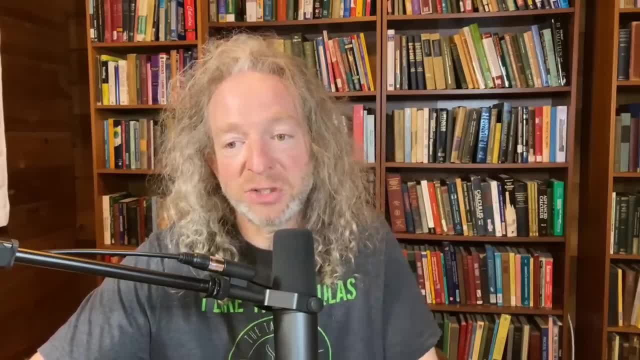 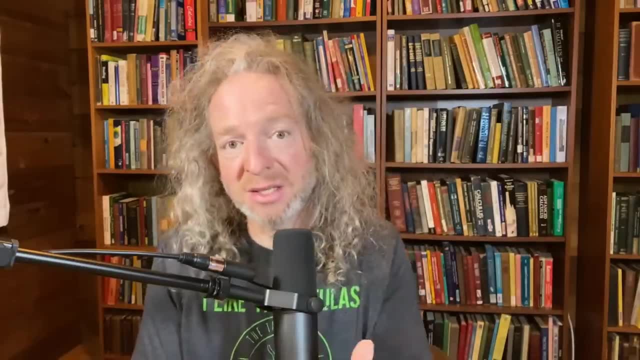 think Amir really nailed it when he said it's the first time I'm encountering proofs in math. Yeah, That's tough For me. it wasn't the first time, So I took two proof writing classes and even then I struggled. So if this is genuinely your first time you're encountering proofs, I would also 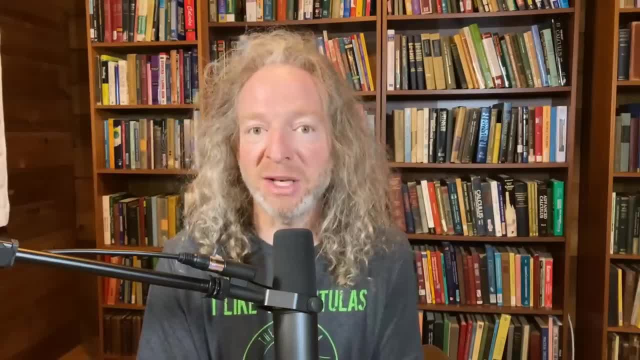 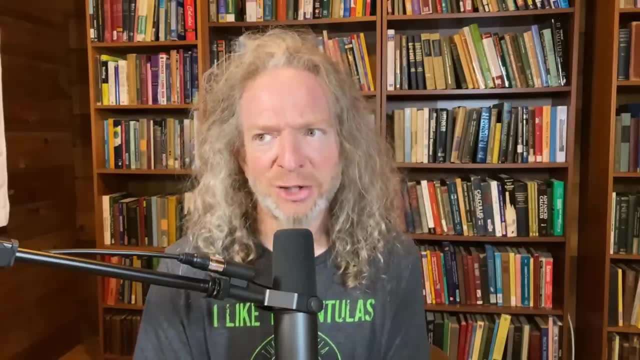 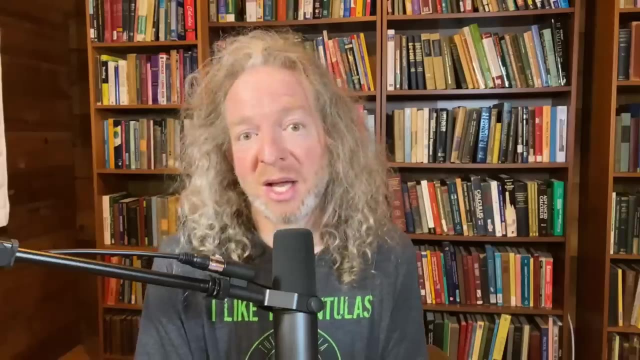 recommend getting a proof writing book. the one by Daniel Vellman, How to Prove It is the one I've been recommending recently to people. It's affordable, kind of. It's small, And I think Vellman does a good job of explaining things many times multiple ways, which helps the reader. 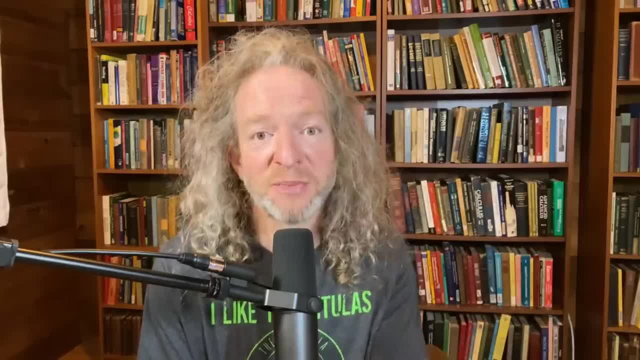 So, yeah, It's a great book. Anyways, if you want to learn math, I should end this video. So let me just say, if you want to learn math, I do have courses. They're on my website, MathSorcerercom I. 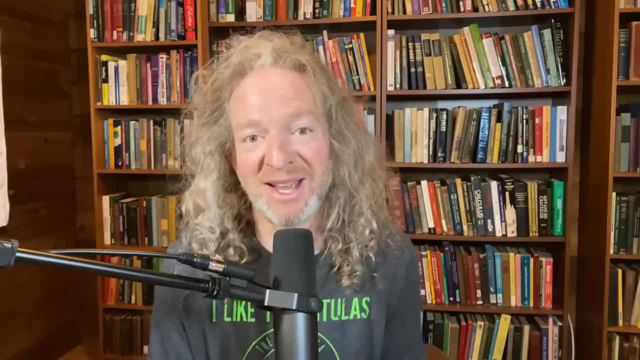 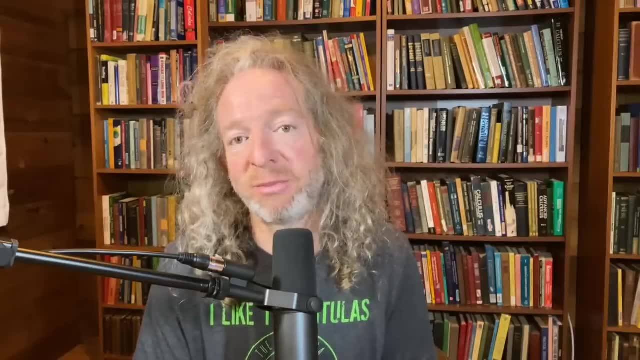 unfortunately do not have a linear algebra course yet. Maybe someday I will make a course on linear algebra. I do have a playlist on linear algebra. You can check that out. I do have some proofs there in my linear algebra playlist. You can check that out as well. And if you're not, a subscriber.